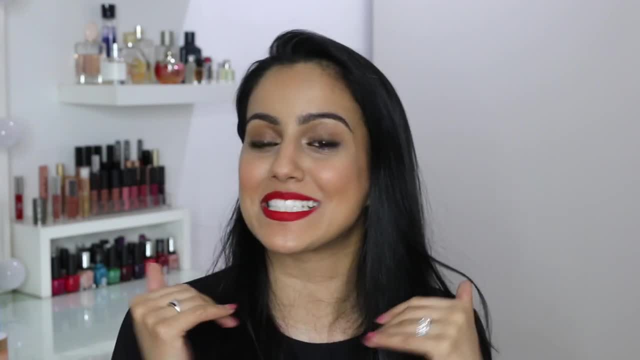 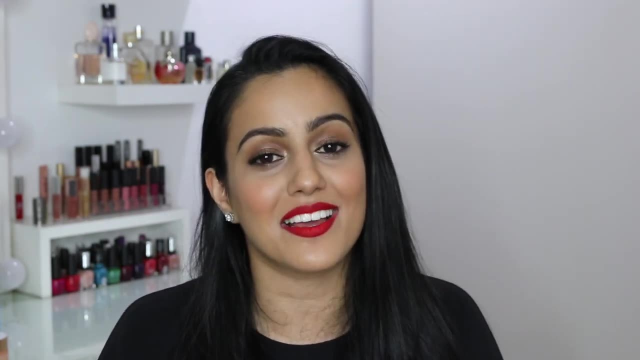 Hello, today's video is going to be all about red lips. I just wanted to get some of my favourites together and share them with you. If you've got a favourite that I haven't mentioned in this video, let me know what it is. I'd love to check that out. I'm sure there are millions of red lips which. 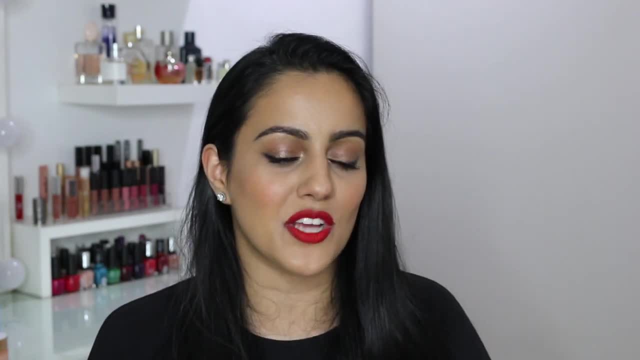 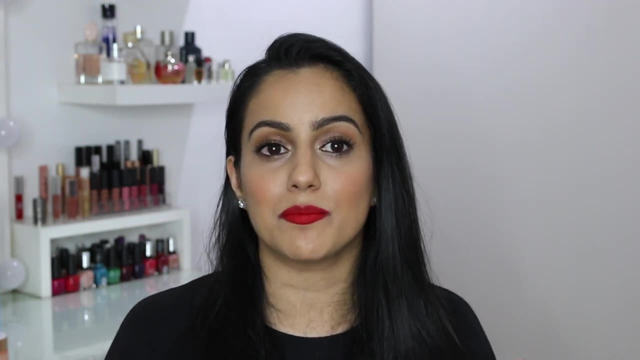 people love and haven't been discovered yet, but these are the ones which I have worn over and over and over again, and I love them so much. So I've done a video on how to apply red lips and I will link that up here, and in that video I give you different ways of wearing a red lip. 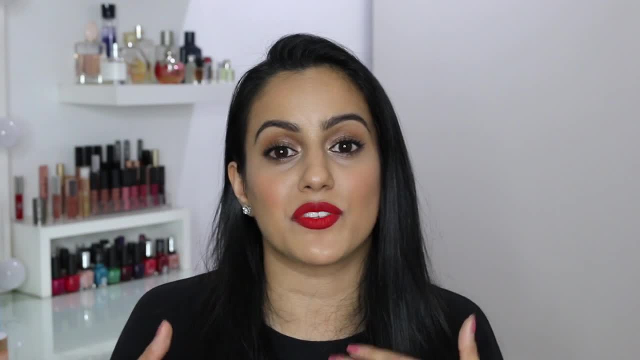 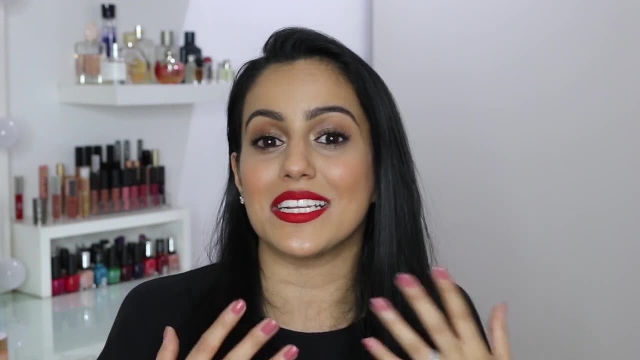 how to apply it lightly and wear it every day for people who don't like to go for the bold look. and if you do like to go for the bold look, like this, how to make it look clean, crisp and just like you've really, really made an effort. So be sure to check out that video. Just want to say 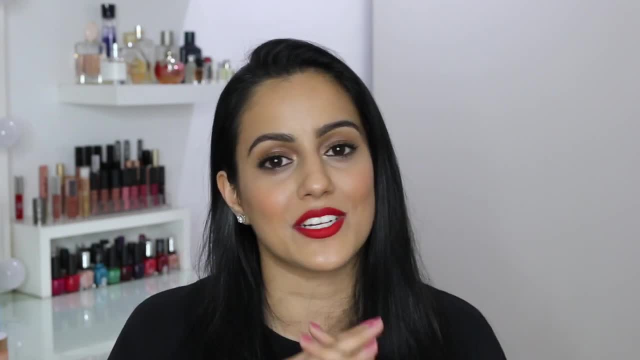 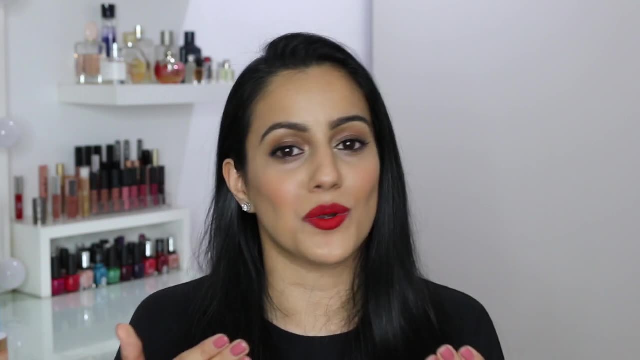 first of all, that everyone's going to have an opinion and everyone's going to have their own taste. so if something I say in this video does not align with your thought process, it doesn't mean that you are wrong. it doesn't mean that I am wrong. it just means we have different views. 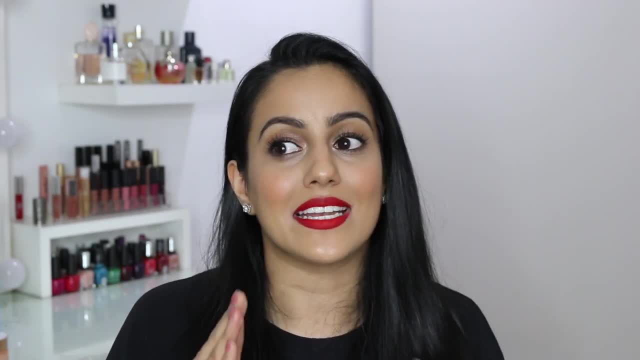 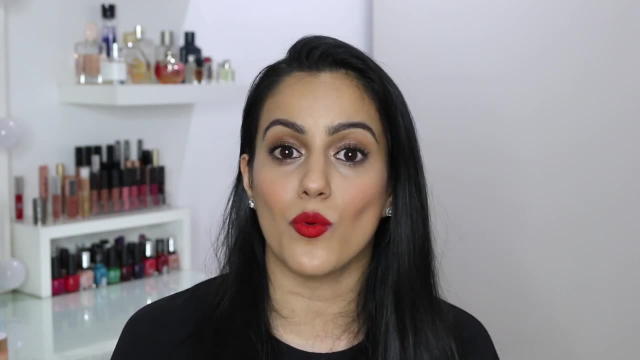 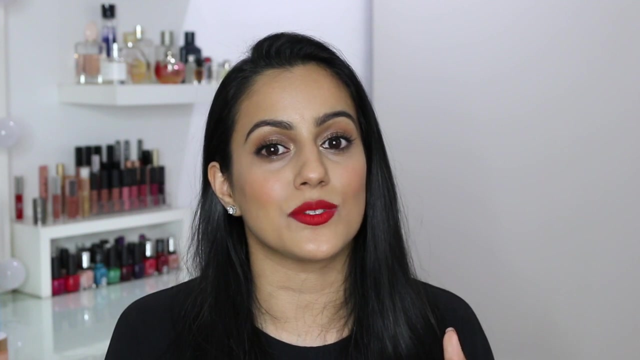 and that's okay. But generally the way that red lips kind of work is, if you have yellow undertone skin, the colours that look really good with your skin tone are ones which have more warmer undertones, so ones which lean more towards the orangier side. If you have a cooler undertone skin, the ones which look 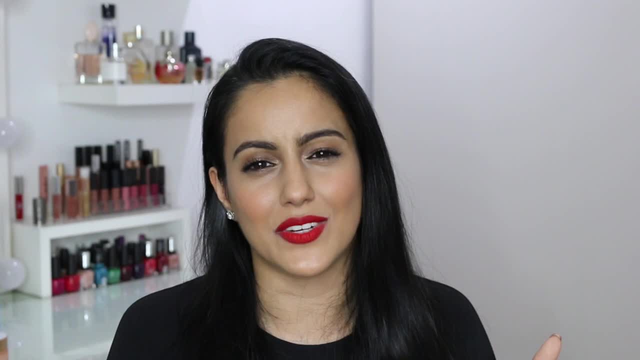 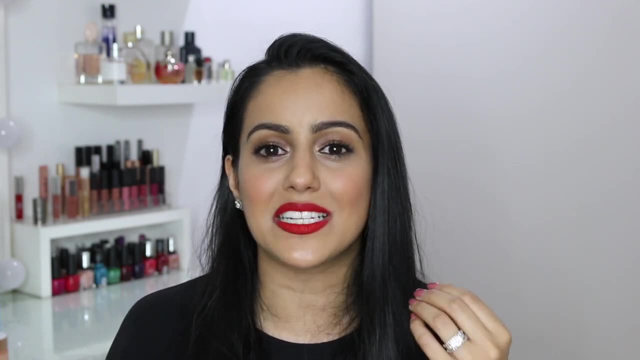 better on you are the ones which have more of a bluey kind of undertone. I personally like it the other way around. I like a cool toned lip on a warm toned person and that's because the cool tones in the lip is going to really pop against the warm tones in my skin and it's going to really make it. 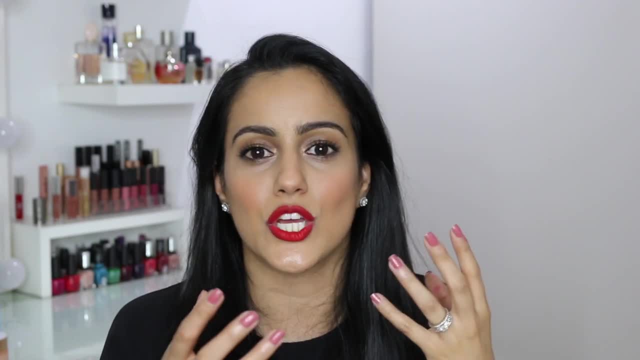 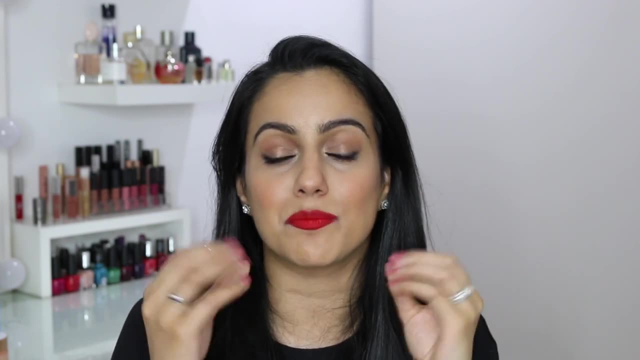 stand out, And the same with cool tones. If you've got a cool undertone on your natural skin colour and you wear a warm toned lip, that's going to be a really good contrast with your skin tone. It's going to make your lips pop and look really, really beautiful. Obviously, you can go with whatever you. 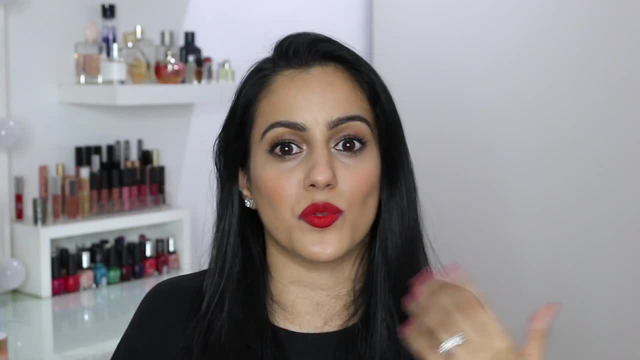 like. At the end of the day, you need to feel good in what you're wearing all the way. You're never going to feel confident going out and rocking your red lips. You'll see in the video that most of my red lips are red lips. They are the ones that I work with the most. I like them the most. I think they're. 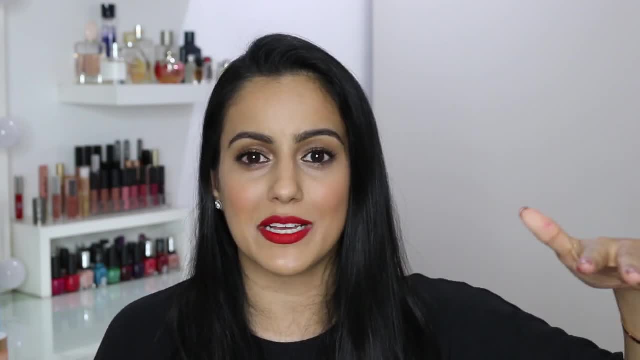 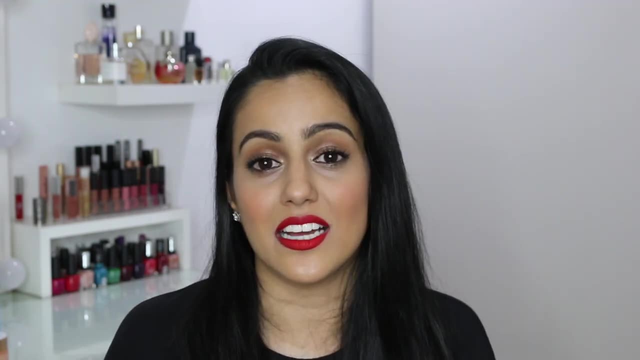 red lips lean towards more of the neutral and polar tone kind of spectrum. I think I have one which is slightly orangey, but I don't have very orangey undertone red lips. Another thing that I love about blue undertone lipsticks is that they make your teeth appear more white. They just 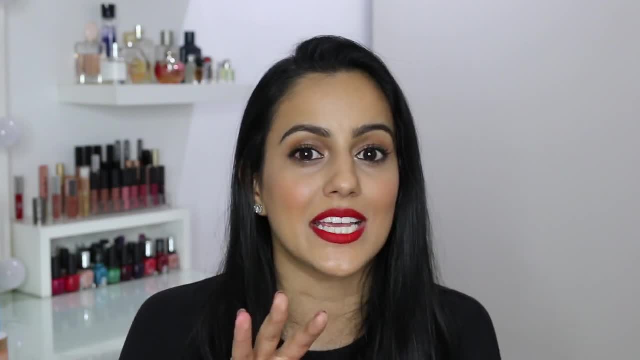 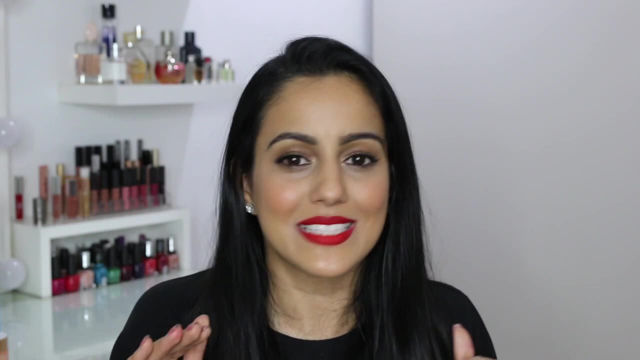 contrast with the colours in your teeth a bit more and make the whiter shade pop more, So it makes your teeth look really, really, really white. I get so many questions on what whiteners I use for my teeth, but I don't use any, and it's especially when I'm wearing a red lipstick, and it's because 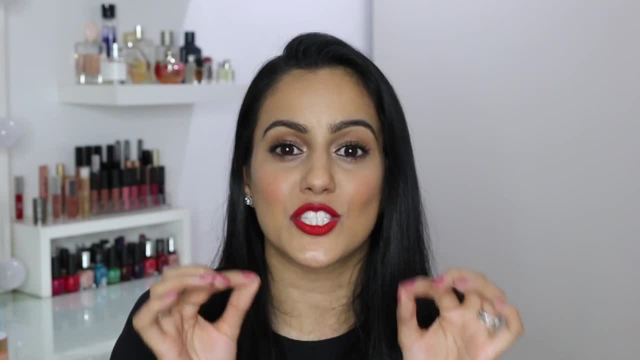 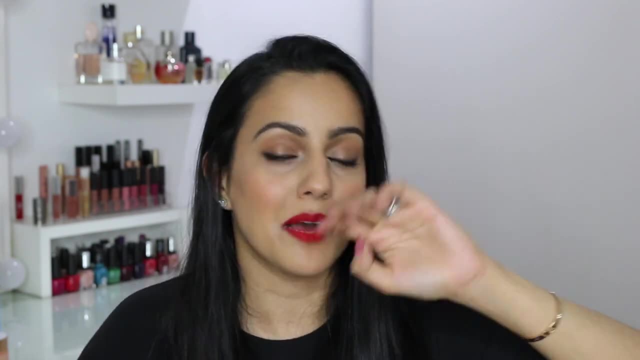 I wear blue undertone red lips and it pops against my teeth, so so well. So that's another thing that I like personally. about blue tone red lipstick. I'm gonna stop talking because I've got so much to say about the ones that I've chosen, so let's get started. The first one I'm going to talk about. 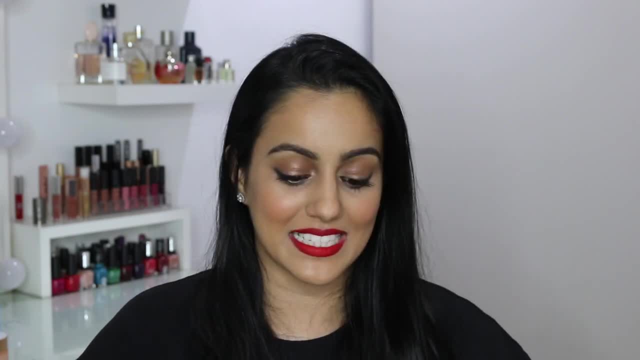 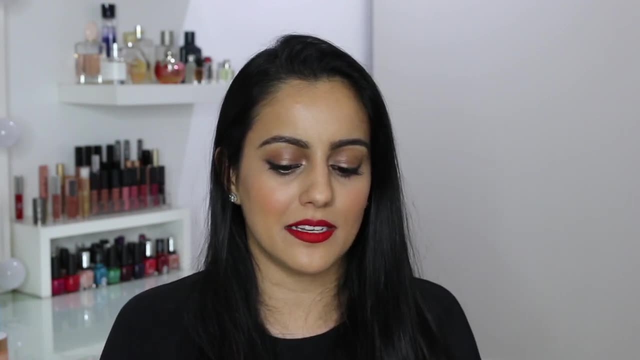 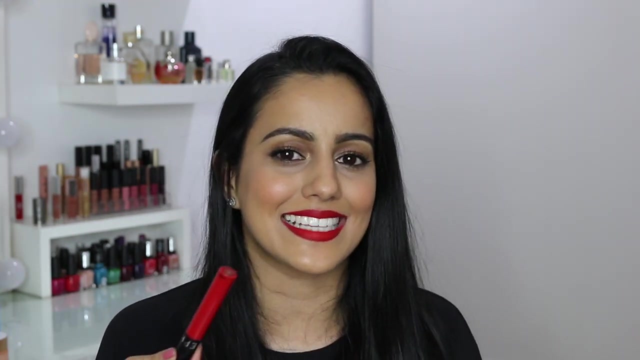 is probably the most underrated lipstick that I have seen online, and I don't know why, because it's such a good formula. It's the Sephora brand and it's a cream lip stain in the colour 01, always red. This is more of a neutral toned red and it goes with any skin tones, from light to medium to dark, I feel. 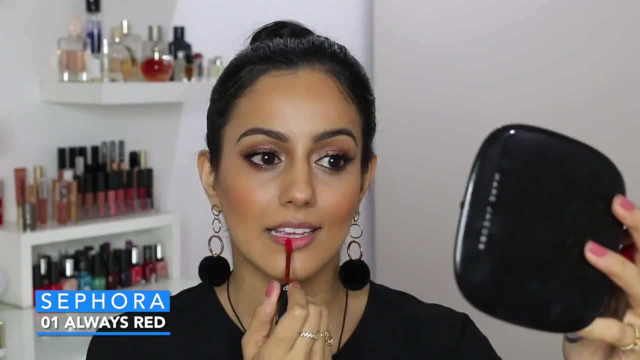 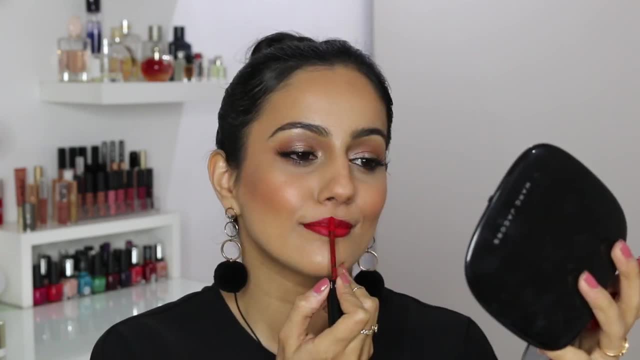 like this pops on every skin tone and there's just something about it. It just looks so good on everyone. I get so many compliments when I wear this and everyone's so surprised that it's Sephora brand. I really love the formula of this as well. Although it's matte, it's not a drying kind of. 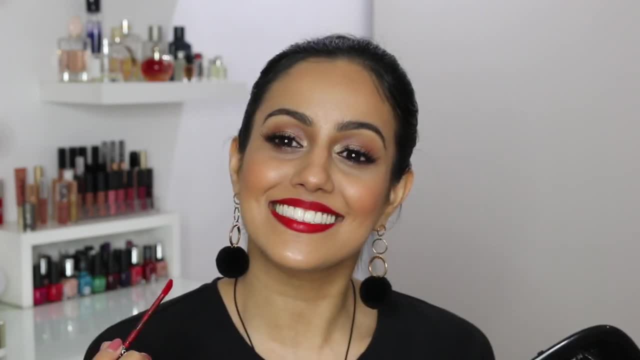 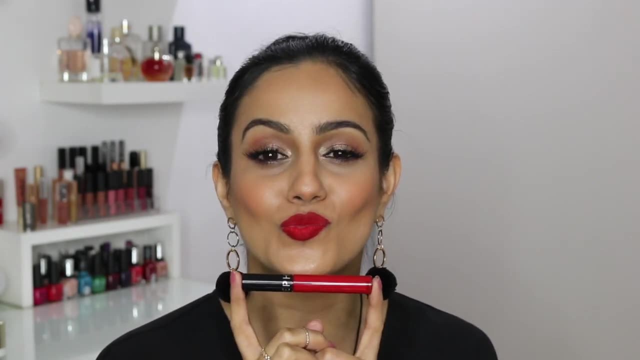 matte. It has a slightly whipped texture to it, kind of like the NYX soft matte lip creams. It's really comfortable and a long-lasting formula and it's so easy to apply. It's not going to accentuate any of the lines in your lips. It's transfer proof, so it's not going to. 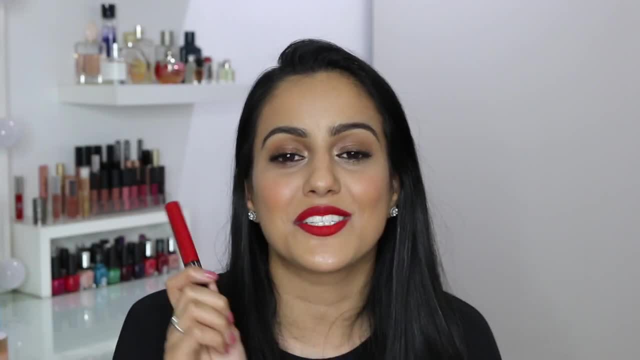 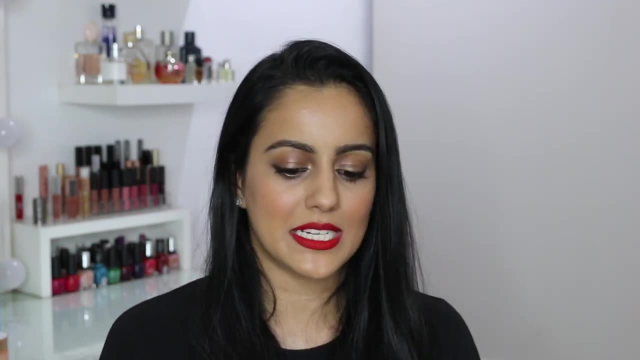 transfer onto anyone and you can go and give some love to the person that you want to give love to, because it's not going to be any sides. That was a bad influence. Don't do that, Don't do that. Next, I want to discuss the NYX lip smacking fun colour and this is in the colour 511.. This is a 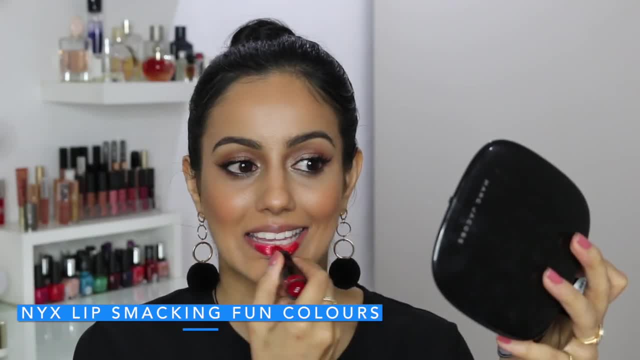 really nice drugstore red lipstick. It's a neutral pinky, rosy red and it's got a really nice satin hydrating formula. So for those of you who don't know, this is a pretty good lipstick because it's very hydrating, It's very hydrating, it's really bright, it's very hydrating and it's really 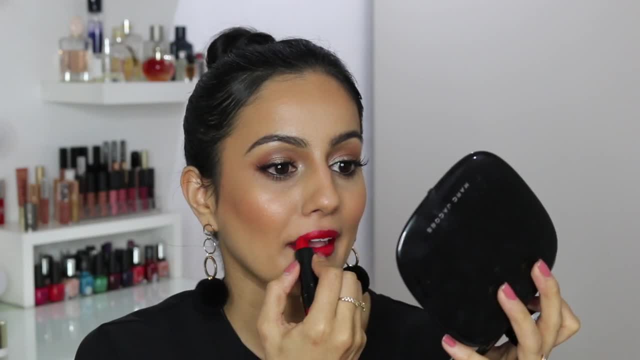 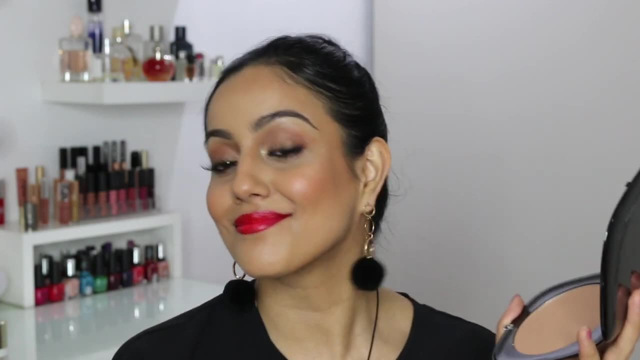 those people who don't like matte formulas, this is probably the one for you. it's a normal lipstick, so you can get all the use out of it. you can put it on your lips as a stain, you can mix it with a balm, you can wear it full on, you can put it on your cheeks, you can put it everywhere. it's really. 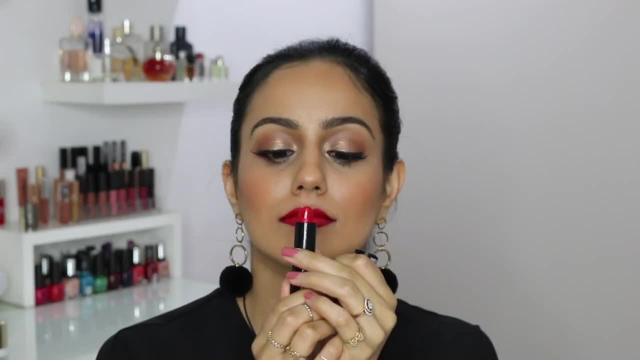 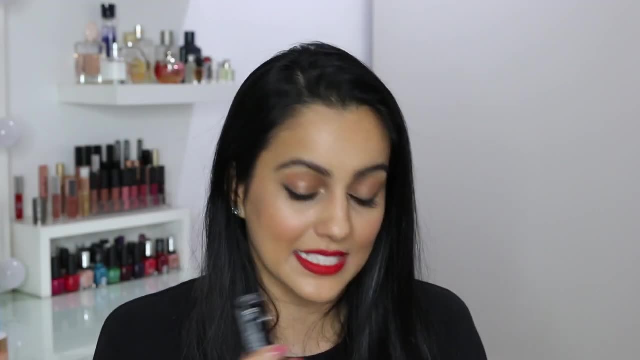 really comfortable, however, saying that it's not as long lasting because it's a normal lipstick. but if that doesn't bother you, it doesn't bother me. i don't see why it should bother anyone. you can just reapply your lipstick. this is really easy to apply. that's why i like it, because, although 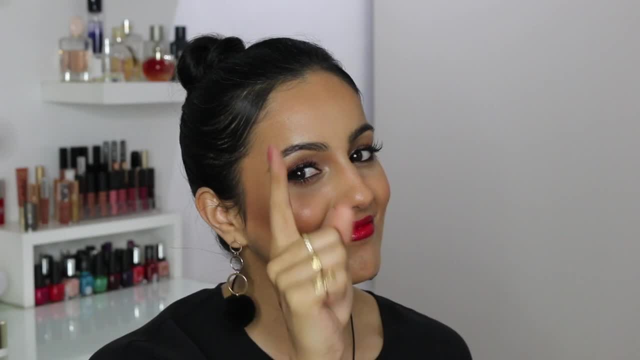 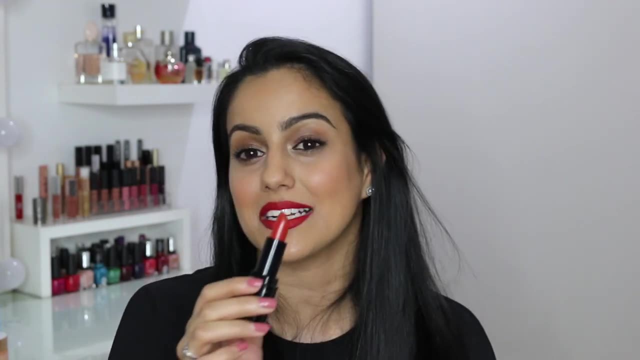 it's not long lasting. it's not going to botch up your lips if you reapply them. another thing is, this is not transfer proof. the next one i want to talk about is this color from colorect. this is a local brand in the philippines. it's not your typical red. it's more of a brick red. it's so. 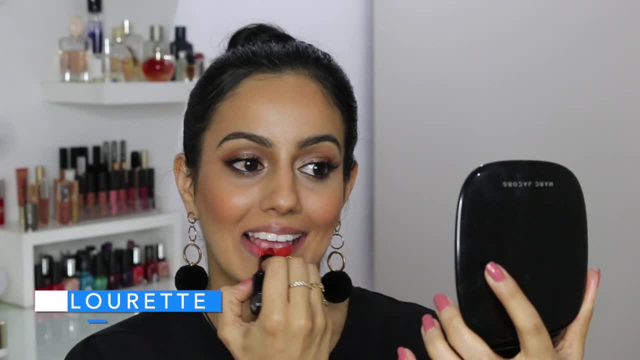 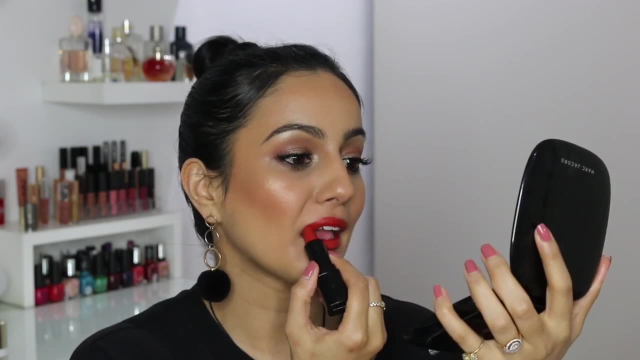 pretty and a really nice alternative for people who don't like going for such a bright, vibrant red. you can go for something like this. it's got more of the orangey and warmer tones in the red and it's a satin finish so it's really really comfortable to wear. it's really hydrating. 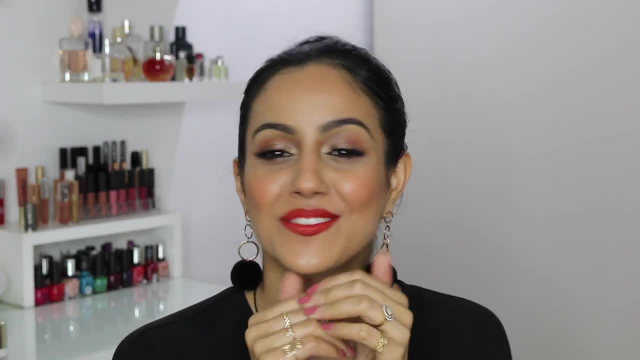 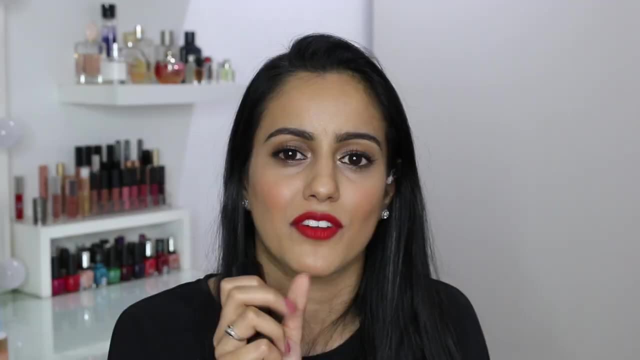 you can go for something like this. it's got more of the orangey and warmer tones in the red and it's it's not long lasting. it does stain the lips, but the actual formula is not long lasting, so you're not going to get the butthole lips, but you will have to reapply it just to get that vibrancy back. 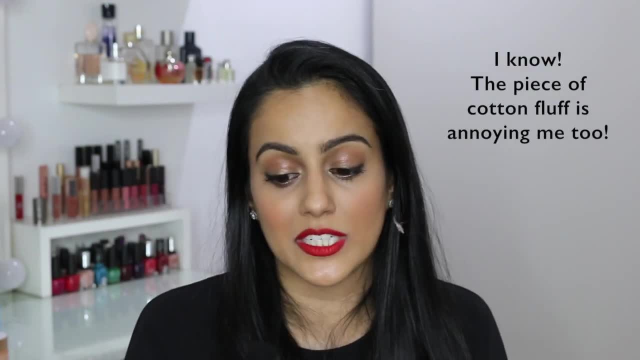 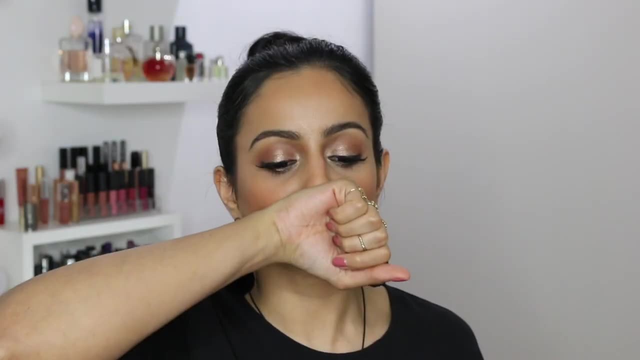 from the color, which is not the end of the world for me. i still really really love this lipstick. again, if you're not the type of person to wear a red lip, something like this would be a really really good option for you. this is also not transfer proof, but i really really like it. 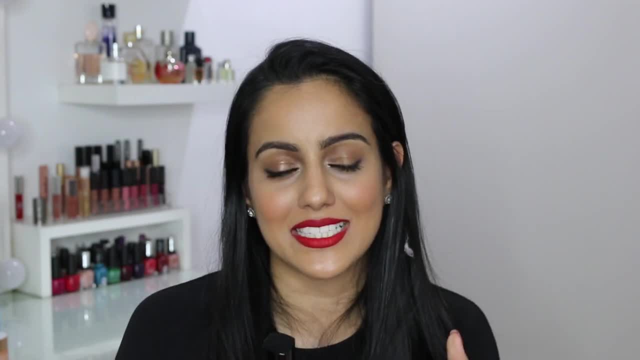 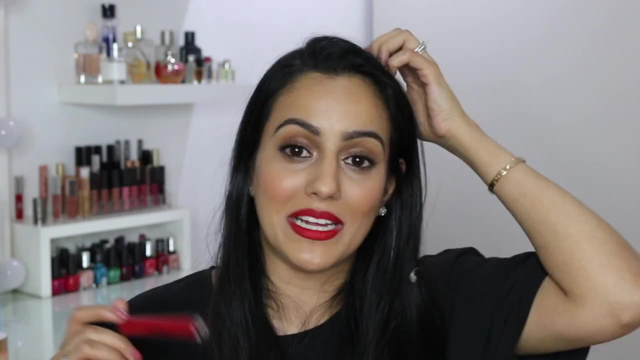 it's such a pretty and unique color. if you're not into the reds, it's just such a nice alternative. the next one is one that you've probably seen me wearing over and over again on my channel or on my instagram, if you follow me there, and that is the stila stay all day- liquid lipstick in the color. 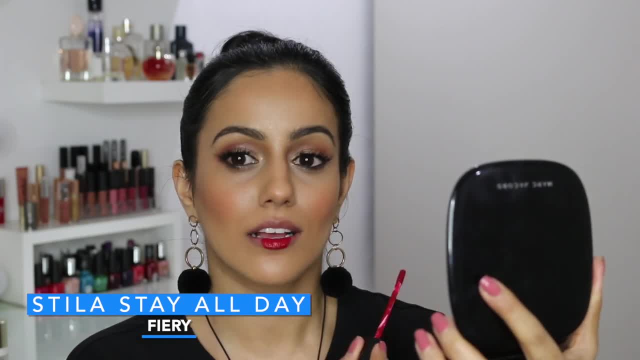 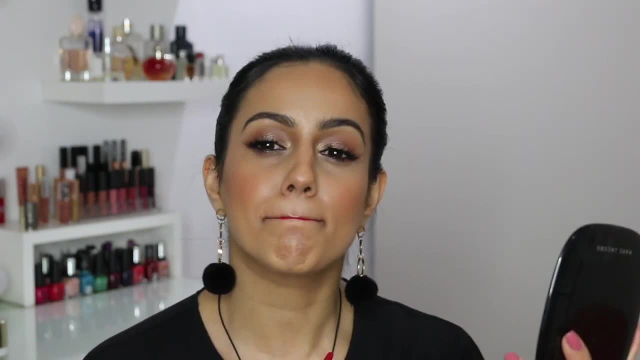 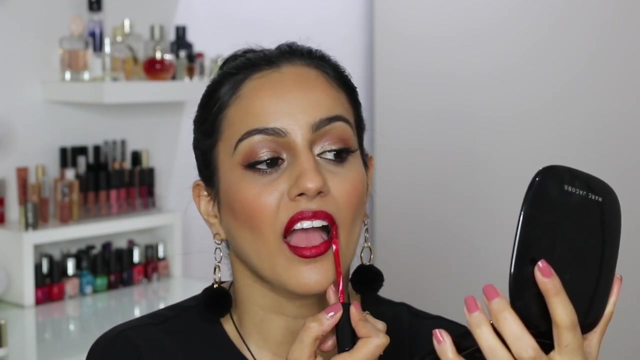 fiery. this is such a pretty red. it's so rich, so deep and looks so velvety on the lips. it's a cool red, so there's a lot of blue tones in it. it is a matte formula, however. it is really really comfortable and it's more like a hydrating matte than a drying matte. these stila liquid lipsticks last forever. 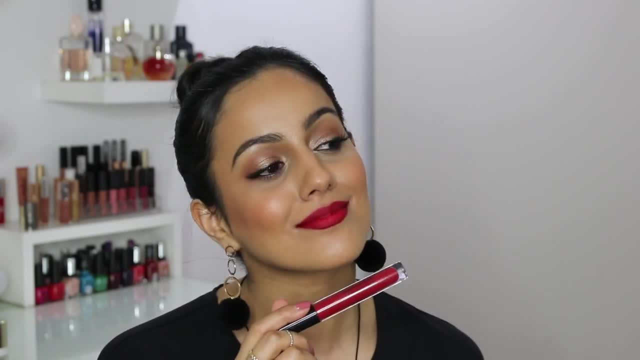 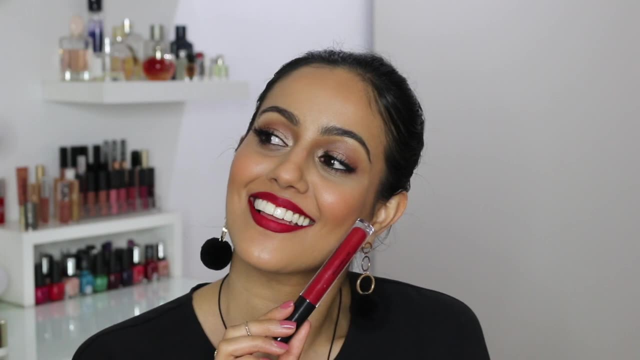 they last until you're done with your lips, and then you're done with your lips, and then you're you want to take them off. so if that's what you're looking for, you might want to check these out. there is another one, i think it's beso, from stila, which is also another popular one, but i 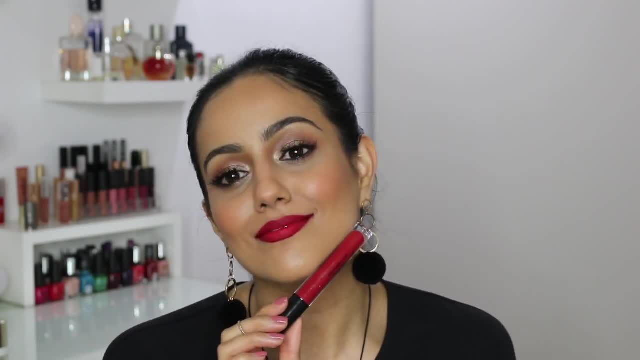 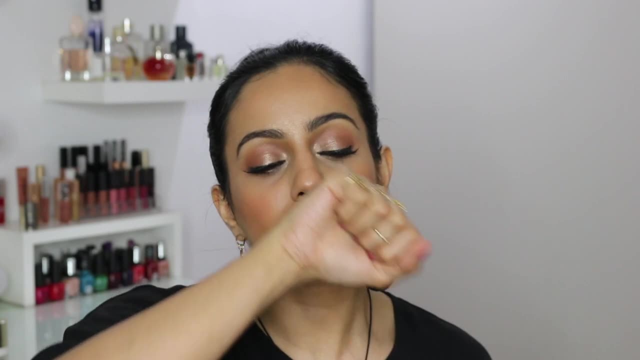 feel like beso and the sephora always red- the one i mentioned before from sephora. this is a dupe for that one from stila. it is exactly the same color, so i went for this one instead because i wanted to try a different formula and i was not disappointed. however, if you like this color, 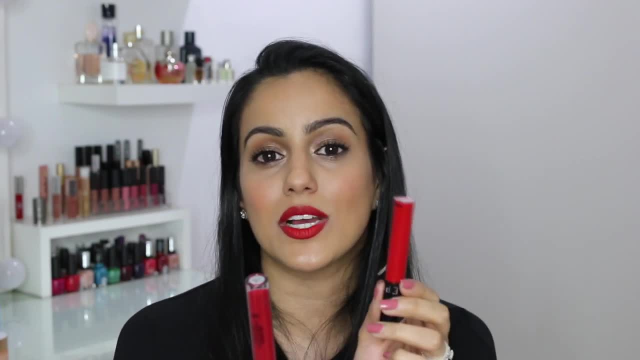 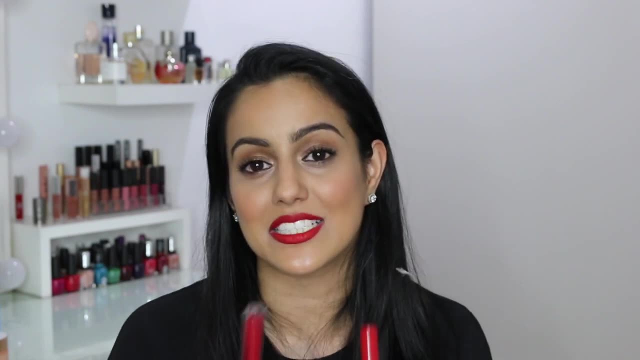 and you like this formula, then i would recommend going for beso. if you want to try the beso for a cheaper price, go for this. if you want to try another color from the stila collection, try fiery. it's just a really, really pretty color and it goes really nicely with all. 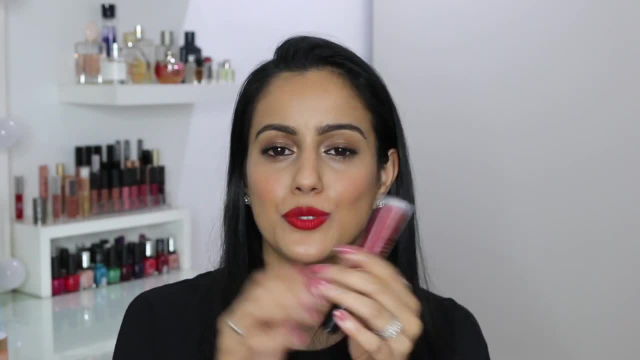 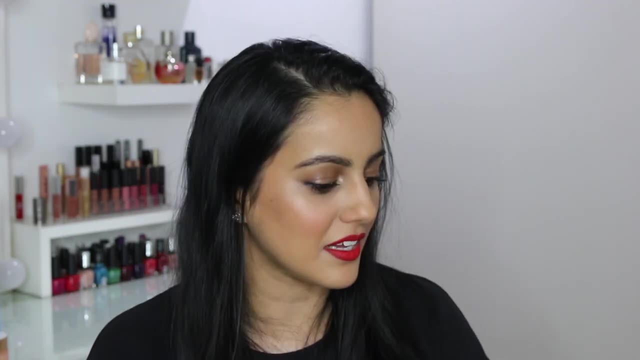 skin tones, and that's one of my favorite things about this. i love the applicator. it's not too stiff. it makes it really really easy to apply the lip. it's a really easy texture to work with. what is this piece of fluff? i had it her whole time. next red lip is probably already. 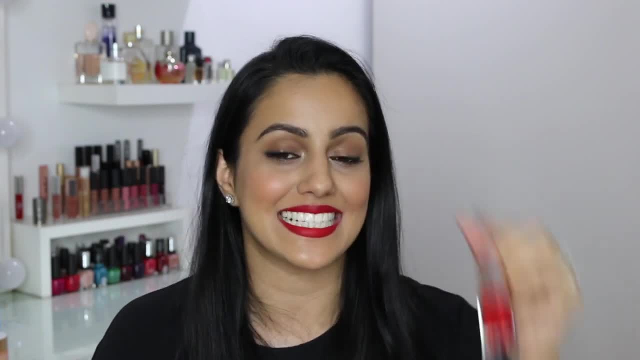 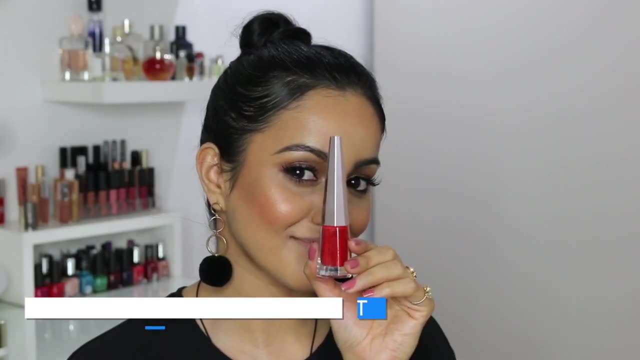 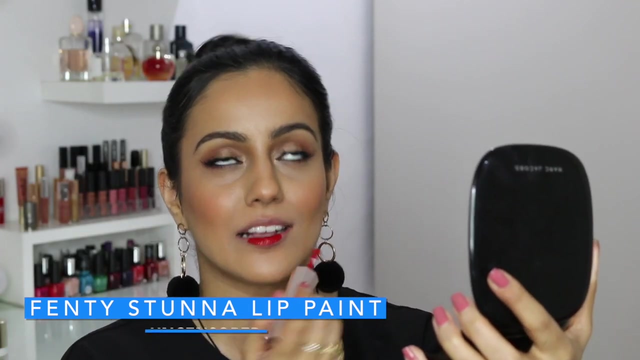 in everyone's makeup bag, especially if you're a makeup lover, and that is the fenty and feta scented standard lip paint. this color is so beautiful. this looks so good on any skin tone, on any shade, whether you're dark, you're medium, you're light. it looks good on everyone and i feel. 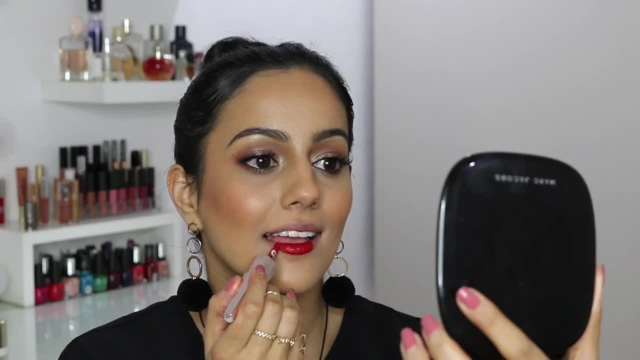 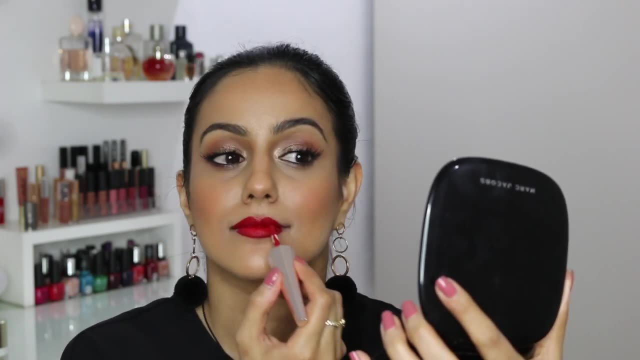 like. that's the essence of the brand. the fenty brand is about inclusivity, so of course this is going to look good on everyone. i was super impressed by this formula. it's really like liquidy and it goes on really nicely. it's comfortable and it is long lasting. however, 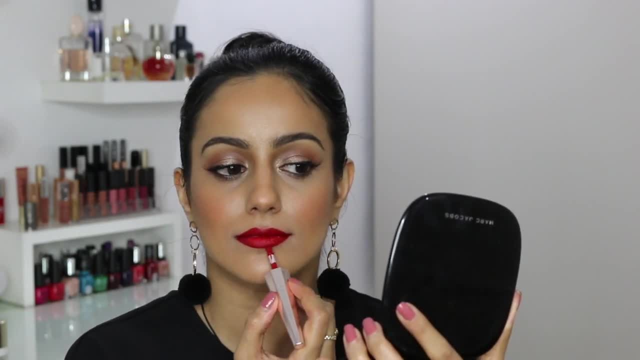 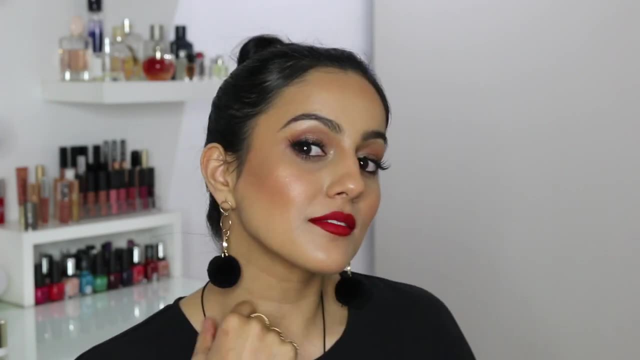 it's not transfer proof. it does get a bit messy. if you are really careless with your lips, i would recommend applying a lip liner, although you don't need to because the applicator is so unique. you get a really nice sharp line. i feel like on me- i haven't heard this anywhere else, but on me i feel like it kind of. 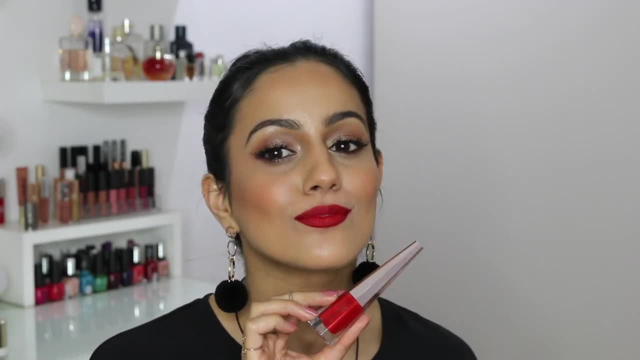 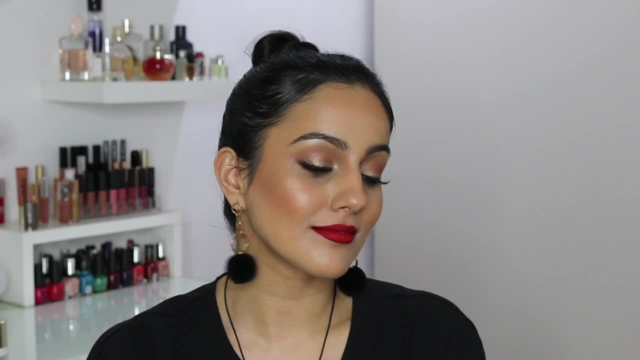 frays at the edges, so i would personally go in with a liner anyway, because i really love this formula and i don't want it to look untidy. i like a really sharp red lip, especially if it's going to be this vibrant and this pigmented. i love it to be really, really sharp. 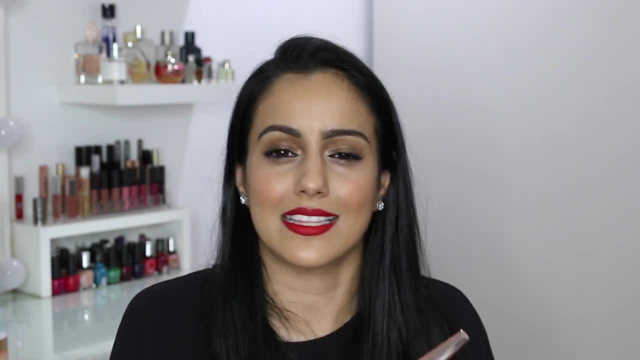 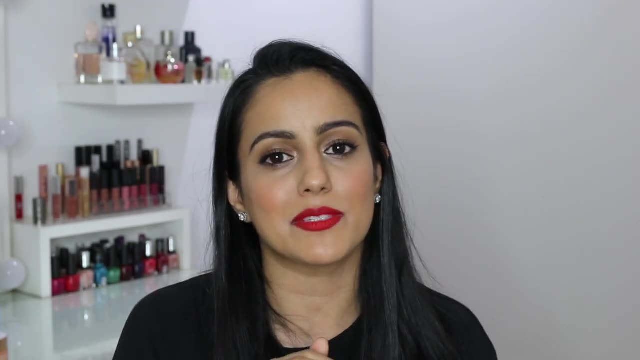 the pigment is just next to none. i've never seen anything like it. if you haven't tried this, give it a go. you won't regret it next. this has been one of my all-time favorite red lipstick. it's been in my professional kit, it's been in my personal kit and i have used this to the boat. 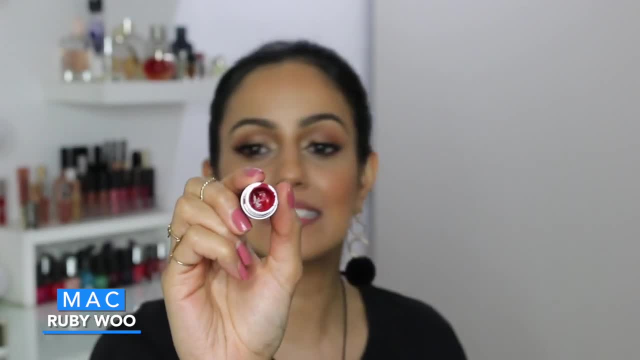 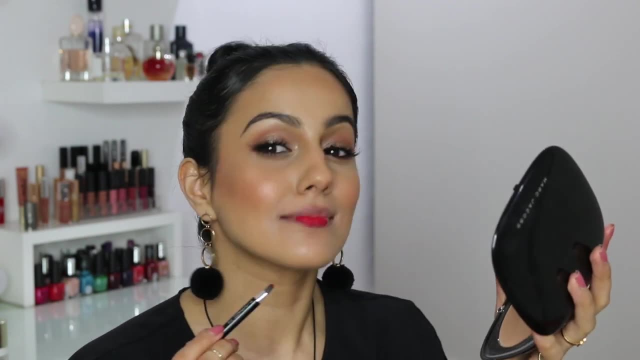 there's literally nothing left. i'm just scraping the sides. i'm waiting to get a new one, because i love this formula. it's like a velvety, retro kind of matte formula. it's so different to the other matte formulas that i have in my collection i can't describe it, if you've tried. 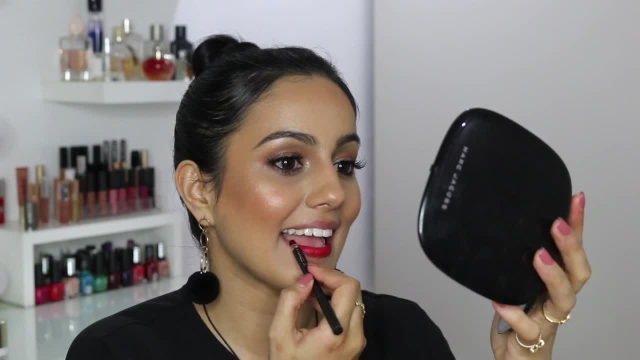 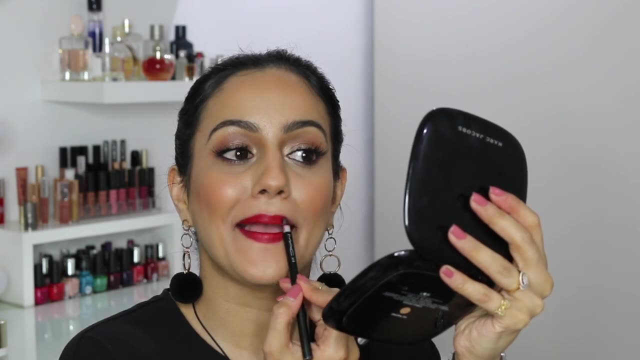 ruby wool. you know what i'm talking about. it's a classic color, a classic formula. it needs more of the neutrally blue kind of red, and that's what i really loved about it. it goes with any skin tone. it looks good on everyone and i keep it in my kit specifically for that reason, because if anyone 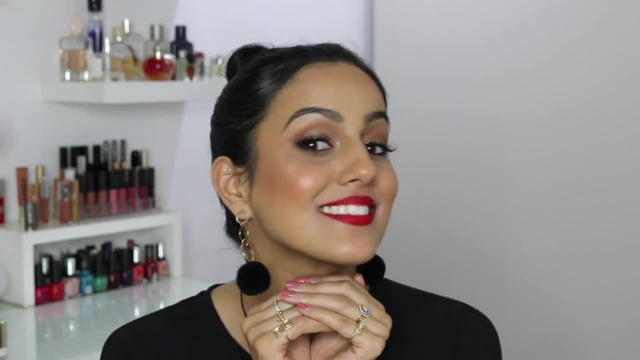 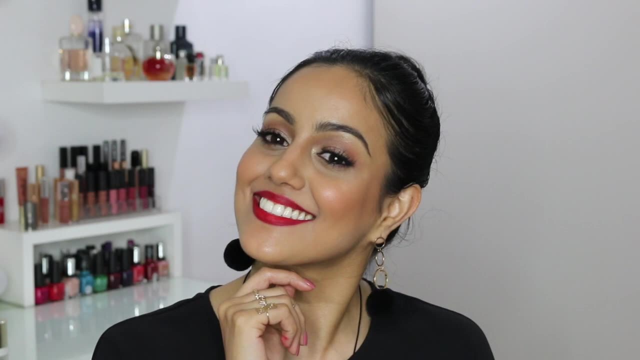 wants a bright, vibrant red lip that is going to look great. i would highly recommend this one. if you don't like a matte formula, you can just top it off with a gloss or something. it can be a clay gloss, it doesn't have to be a red one, but it's going to look really pretty however you apply. 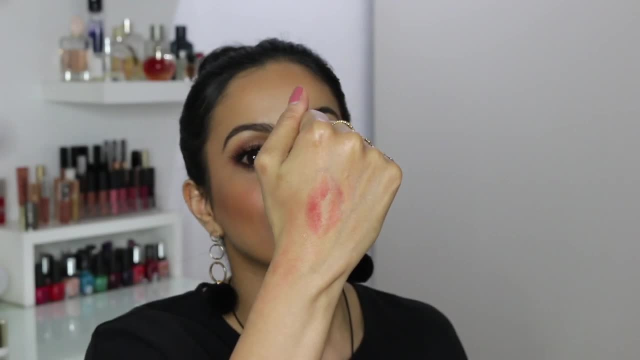 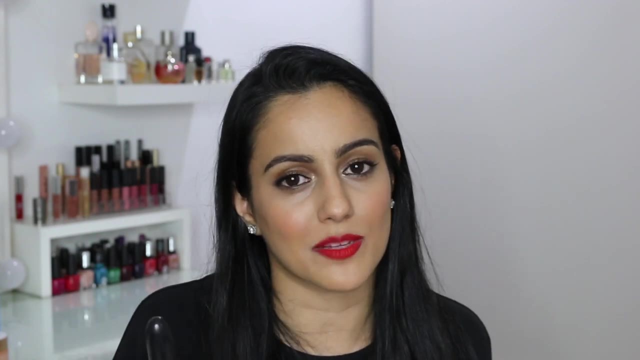 it. it's really comfortable, really long lasting. however, it's going to give you a really nice finish. it's not transfer proof. in my experience, i learned that the hard way because i don't really like to eat. when i go out, i'm always snacking on something. i've always got something in my hand. 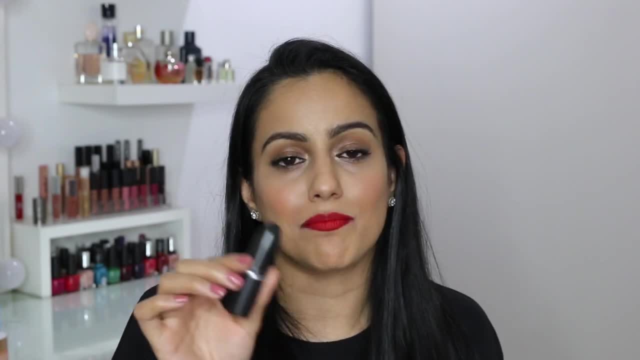 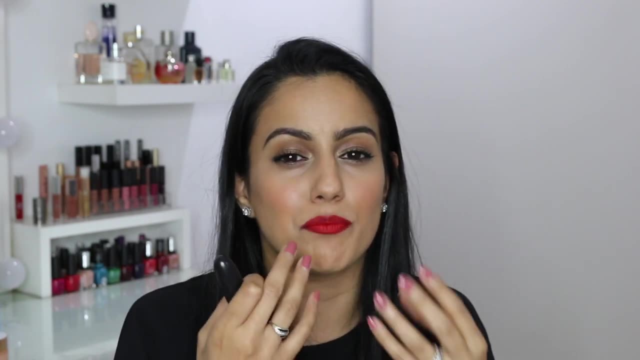 so yeah, that's how i learned that this was not transfer proof. even though it's a matte formula, it is really, really easy to reapply. you can put it on and if it like wears off in the middle, you can reapply. it's not going to botch up in the middle of the process. lastly, i want to talk about this: 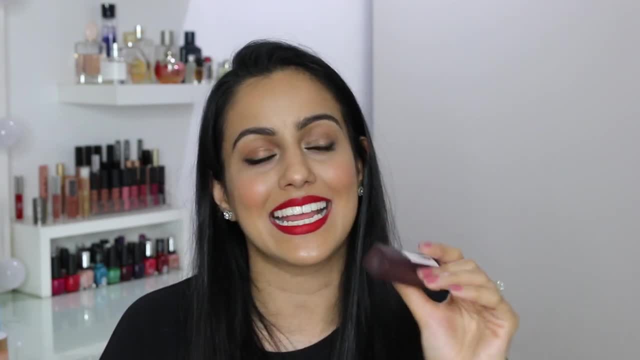 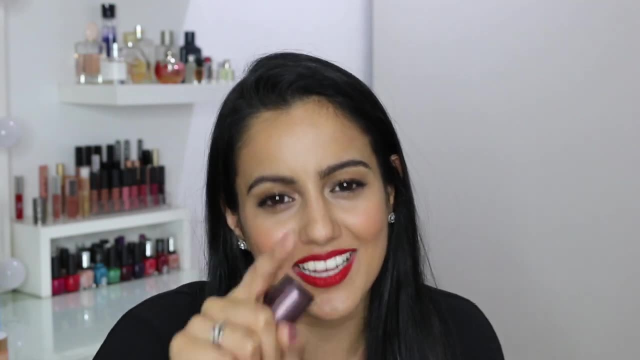 one. this is from maybelline. this is the color, divine wine. it is just that it's divine darling for charlotte tilbury impression. even though i have a british accent that sucked for me. this is such a unique color and it's such a different take on a red lip. it's really, really deep. it looks so. 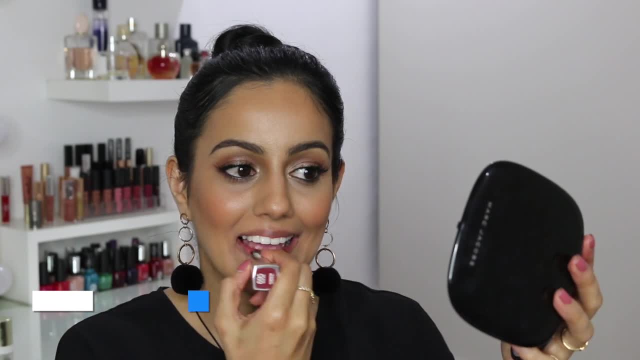 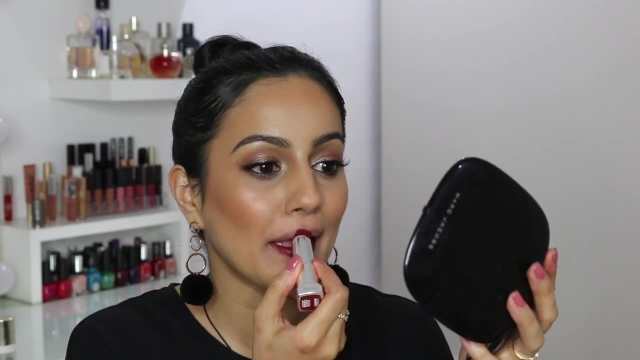 good. this is from the drugstore, and drugstores do really really good lip products. the only problem with drugstore is that their color selection can suck a little bit, but if you find a good color, you're gonna be really, really happy. this is a matte lipstick, but it's a hydrating matte lipstick.